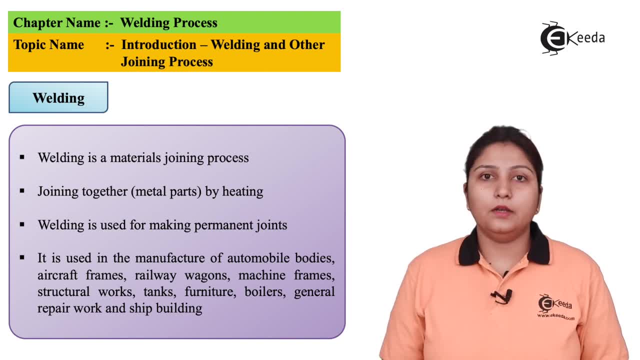 So I'm talking about welding, what is welding and its allied processes. So in welding, what you do is you join two or more than two materials together by the application of pressure, or you don't apply pressure, by the application of heat or heatless. So in this way, two or more metal, non-metal objects can be joined using welding. 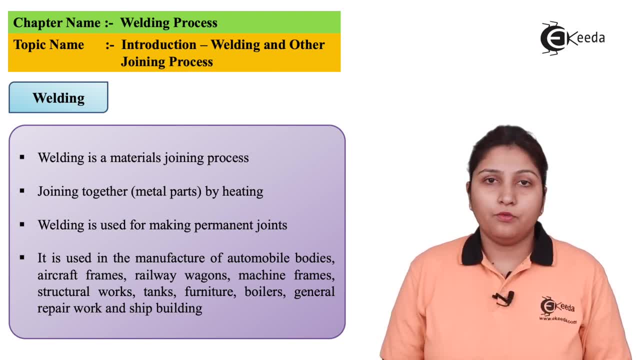 process. So while heating, the temperature may vary from metal to metal. So when the metal is harder or anything like, heating varies with metal. That's what I want to say. So in welding process, what is done? two metals are brought together. 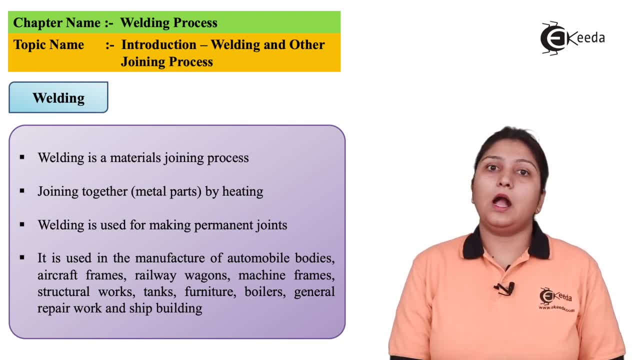 Arc is stuck between them, but that only in arc welding. When we'll go to gas welding, gas is used. When we'll go to other welding processes, other materials are used. So the basic aim of my video is to explain what is welding process and other joining processes. 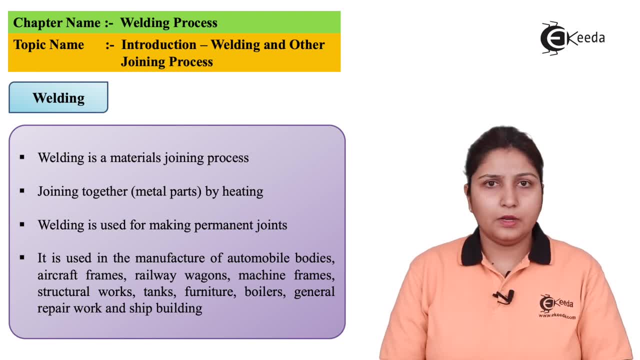 So in welding two metals are welded by welding process, Then the joint is permanent, It cannot be removed, while in case of other joining processes, like if you do it by doing a desive bonding or you do it by riveting, the joint can be removed again unless and until it. 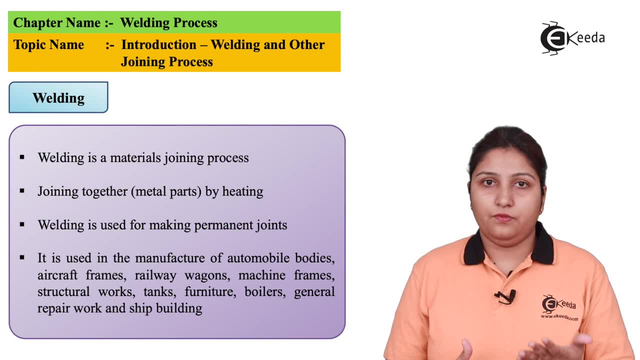 is permanent, Like in case of a desive bonding, if the adhesive is not strong, it can be removed again. So this is the basic process of joining. Okay, So now we are talking only about welding. Weld is permanent, It is joined together. 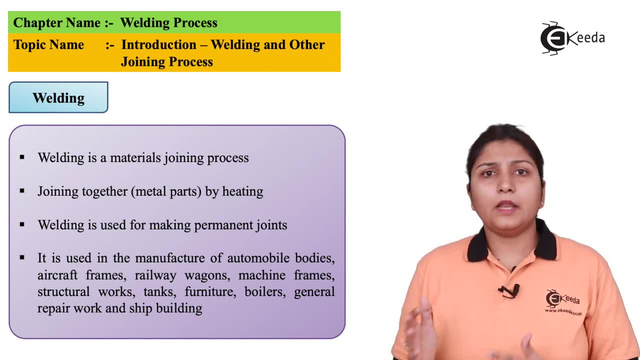 and with a permanent joint. There are many types of joint, like butt joint, weld joint, lap joint, which we are going to see in other videos. So if I'll give some examples or applications of welding, they are used in each and every field. 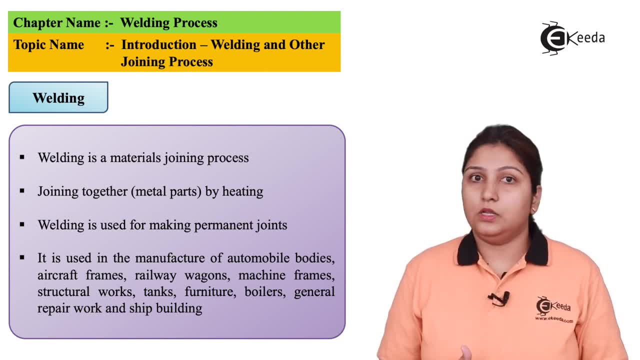 Like, if you want to make an aircraft, if you want to go and work in railways, car, anything. this is the basic thing which I'm talking. If you want to weld two metals, you can do it by welding. If you want to weld two metals, you can do it by riveting.